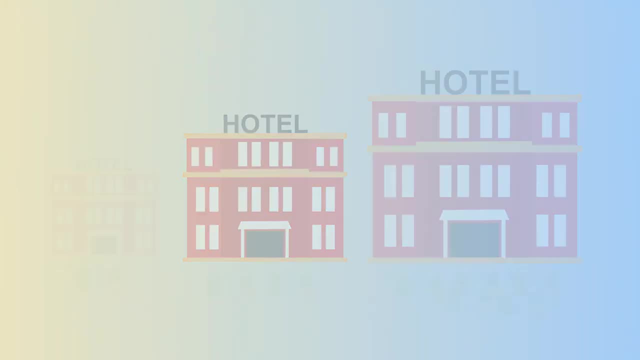 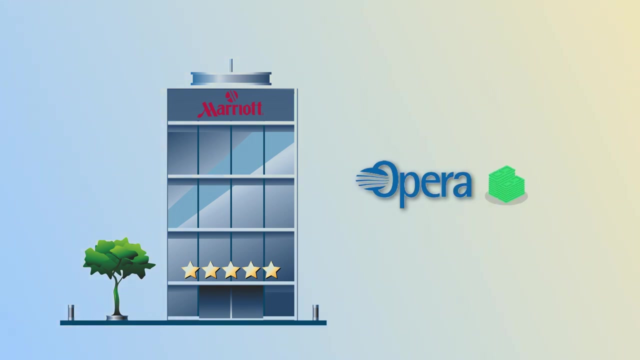 your hotel and the budget you have put aside for a PMS. The Marriott utilizes Opera, which is the industry standard for property management software. With that, of course, comes a higher price that most small-to-medium-sized hotels can't afford. Some hotel chains spend money to develop. 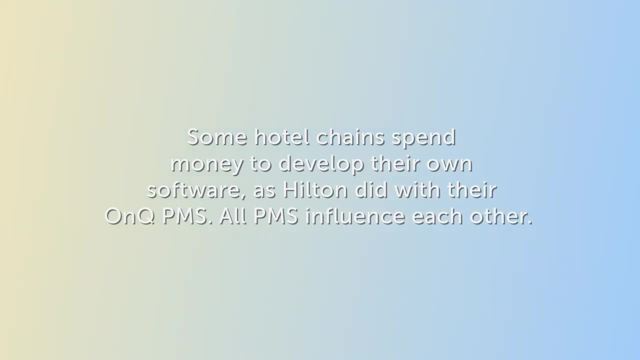 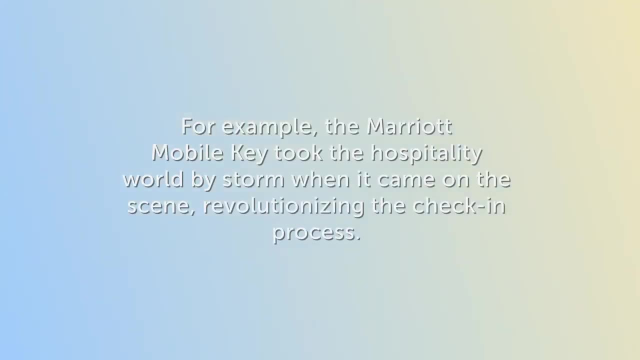 their own software, as Hilton did with their ONQ PMS. All PMS influence each other. For example, the Marriott MobileKey took the hospitality world by storm when it came on the scene, revolutionizing the check-in process. With a MobileKey: guests could check in on a mobile. 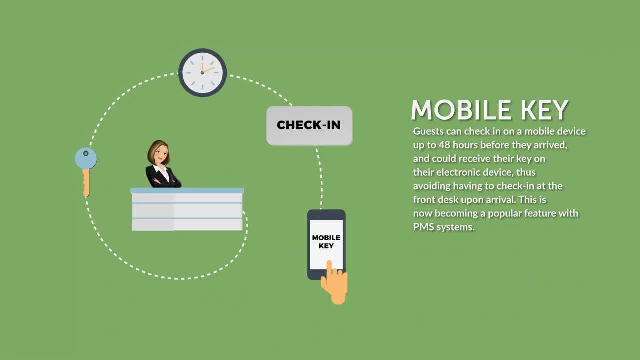 device up to 48 hours before they were able to get to the hotel. The Marriott MobileKey is a feature that allows hotel managers to check in before they arrived and could receive their key on their electronic device, thus avoiding having to check in at the front desk upon arrival. 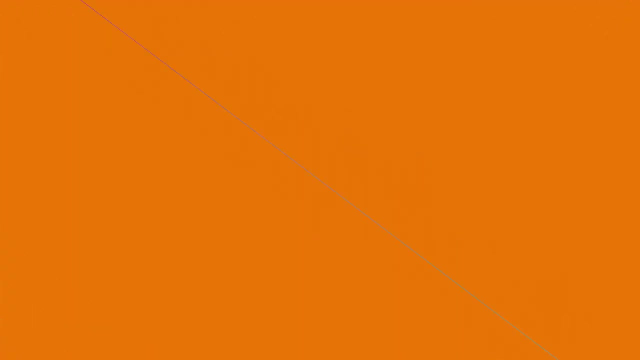 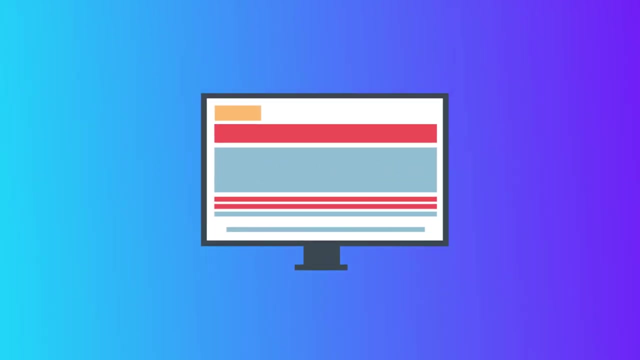 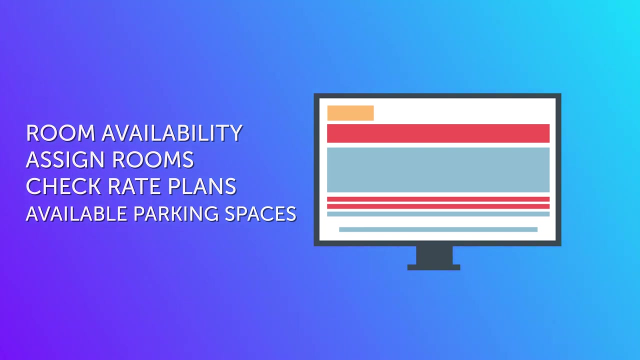 This is now becoming a popular feature with PMS systems. Speaking of features, there are many more that I've yet to mention. The Reservation Management System makes it easier for hotel staff to view room availability, assign rooms, check rate plans and view available parking spaces. You could also easily keep track of guest bills assign. 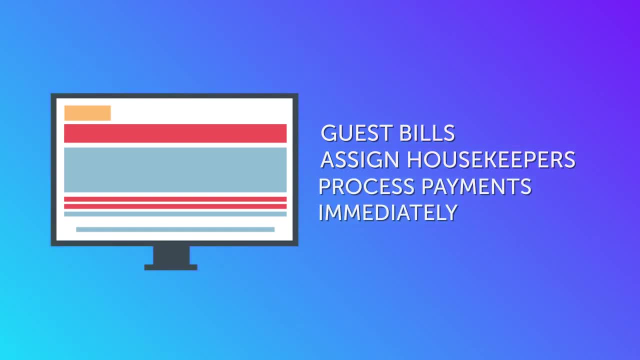 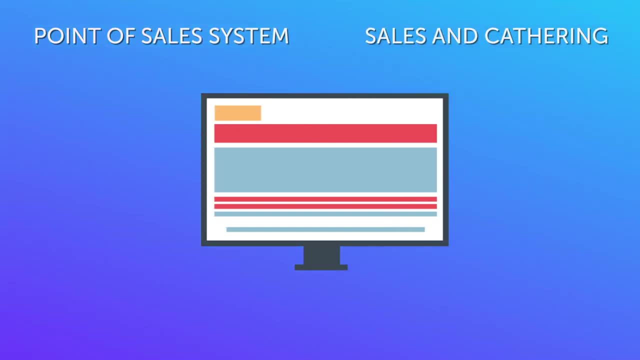 housekeepers to each of the rooms and also keep track of guest bills. And, as previously mentioned, the software connects to every department of the hotel, such as the point-of-sale system, sales and catering, pay TV and compliance reporting. Simply put, property management software is the lifeblood of your hotel. 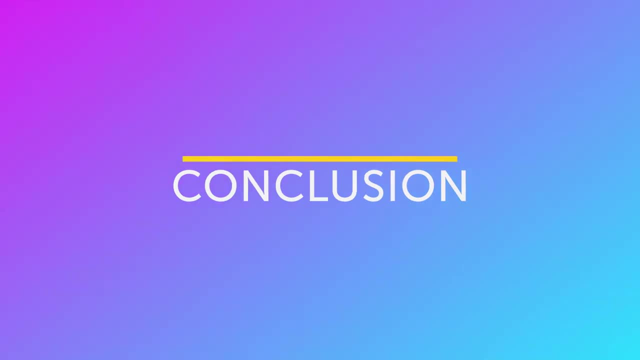 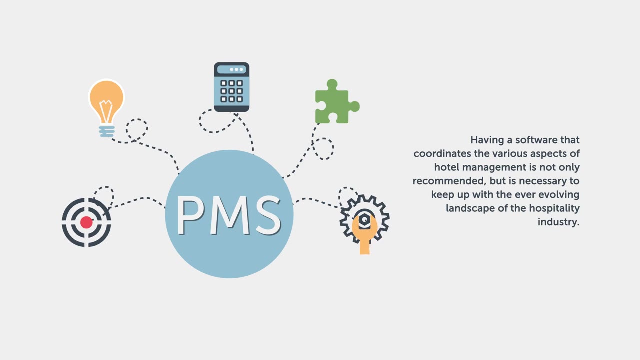 Property managers should purchase the PMS that best suits the needs of their business. In this day and age, having a software that coordinates the various aspects of hotel management is not only very important, but also very important. It's not only recommended, but it's necessary to keep up with the ever-evolving landscape of the 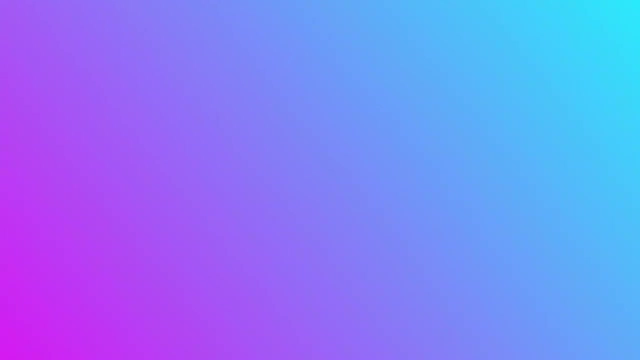 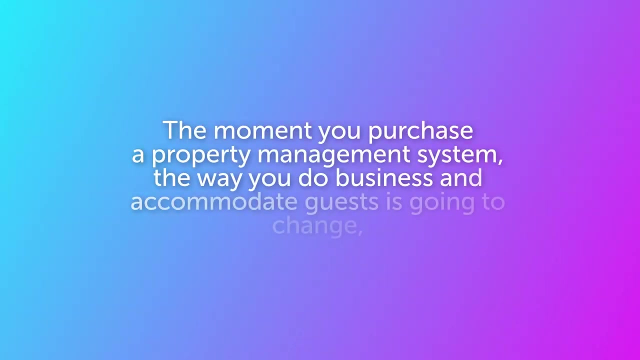 hospitality industry. With online marketplaces such as Bookingcom, Expedia, Airbnb and many other OTAs allowing guests to filter and customize their experience, there is a demand for hotels to follow suit. The moment you purchase a property management system, the way you do business and 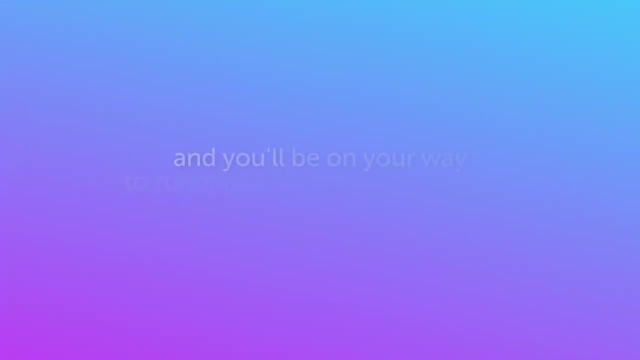 accommodate guests is going to change and you'll be on your way to running a highly successful and efficient hotel. For more information, visit our website at wwwbookingcom.